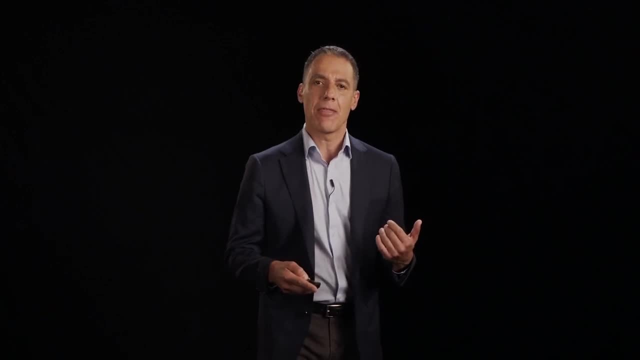 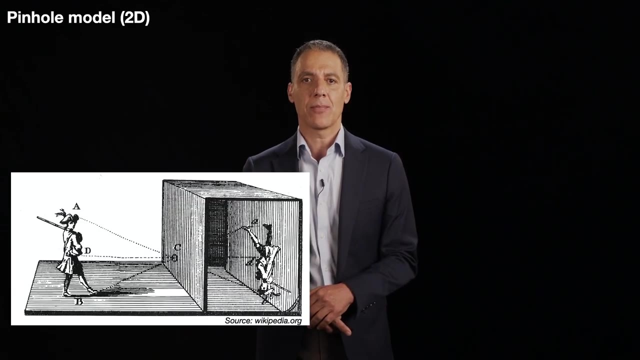 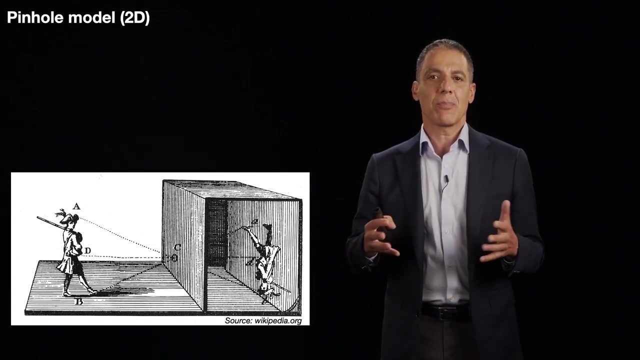 to turn out that we can go back quite a bit and think about really, really simple cameras in order to start to model the image formation process, And what we're going to do is go way far back to the camera obscura. The camera obscura is simply a box with a hole in it And, amazingly enough, 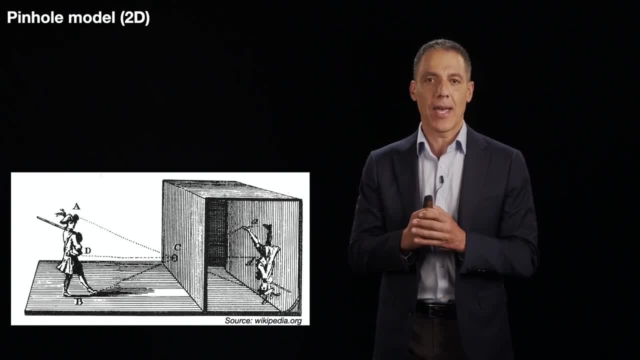 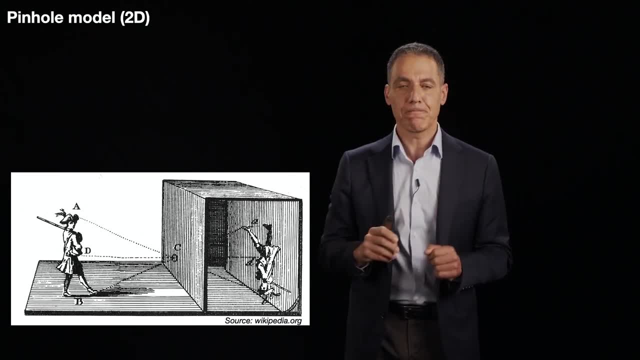 this simple camera, if you want to call it. that is a pretty good model of a modern digital camera, like the one that's recording me right now. So let's talk about this camera obscura. So what is this? This is basically just a box that you see. 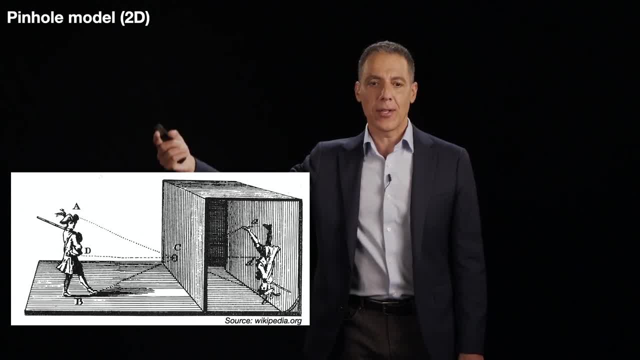 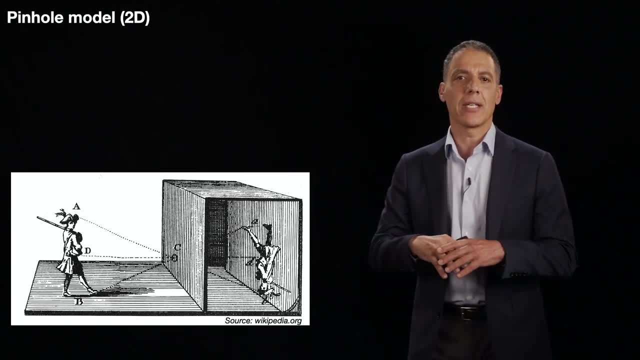 here and a hole in the front where you see those rays coming in, And I've taken off the front face here. but think about it as a sealed box. So think about getting a refrigerator box, cutting a small hole in it, And what's going to happen is that that box with the hole in it is going to be a 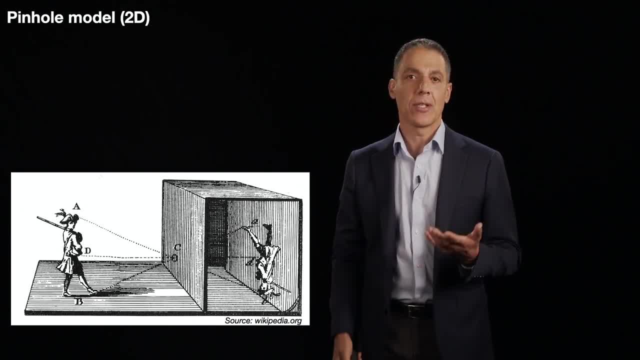 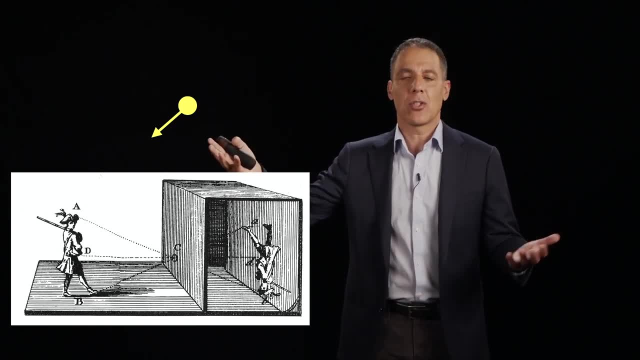 box with a hole in it is going to model a modern digital camera. So let's see how that works. Well, we're going to start with a light. We are nowhere if we don't have light, So we have a light source, which I've drawn right here as a small yellow dot. That light, of course, shines down. 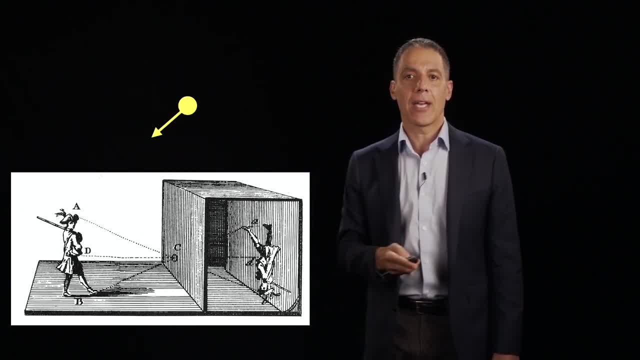 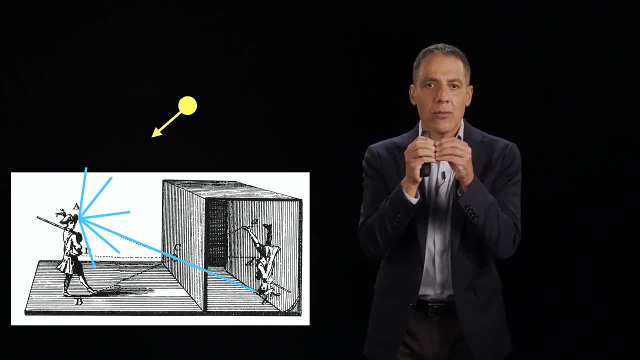 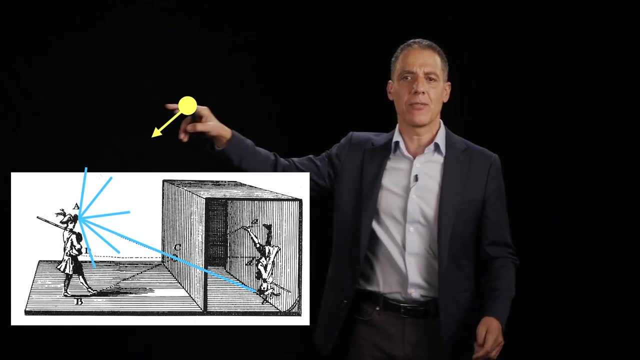 and illuminates the scene that you see over here. And, of course, what happens is that light strikes a point on the person's head, labeled A right here, And light reflects out in all directions. Sometimes it reflects evenly and sometimes it's unevenly. It depends on the actual properties. 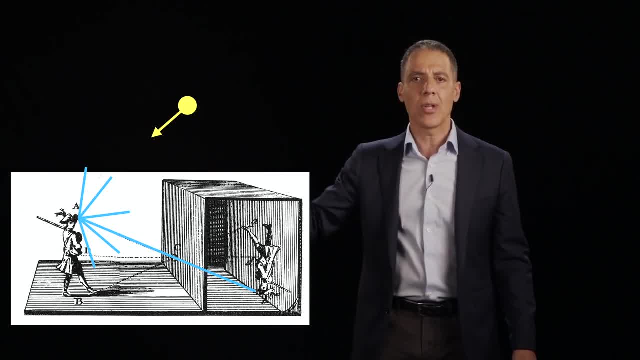 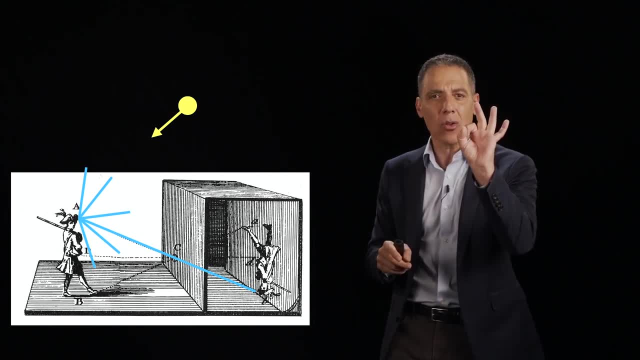 of the surface, But one of those rays, one of those long blue lines that I've shown you, is going to bounce off, reflects off of the sun, bounces and enters that little hole, pinhole in the front of the camera And, by the way, the reason why it's a really, really small hole. 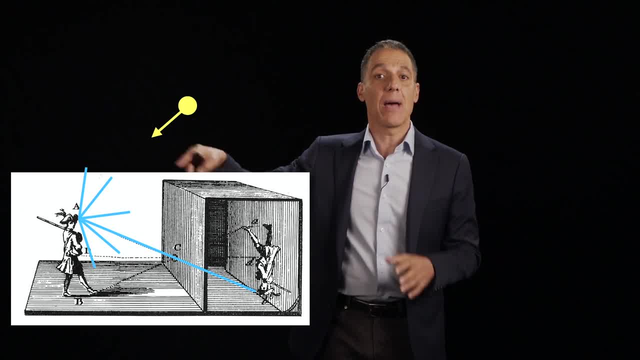 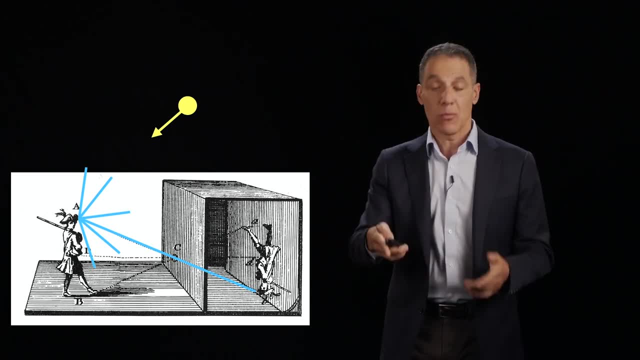 is to allow just one of those rays of light, not more than one. And of course that light ray keeps going and eventually hits the back of the box. And that's what we're going to do here. We're going to get a box right here and we see that point, A mirrored or image, there, And now we repeat that. 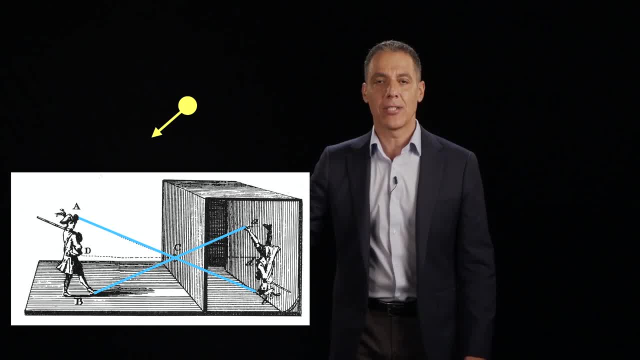 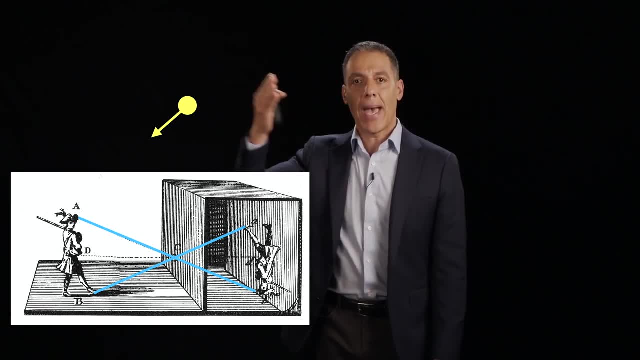 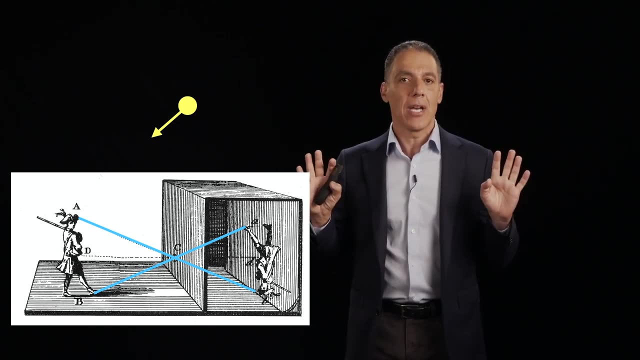 process. And so now the light shines down, hits, say, the foot. That's point D. Single ray comes out, goes through the pinhole and strikes the back of the sensor. And we do that over and, over and over again and we get literally an image. And this is I'm not kidding. You can get a. 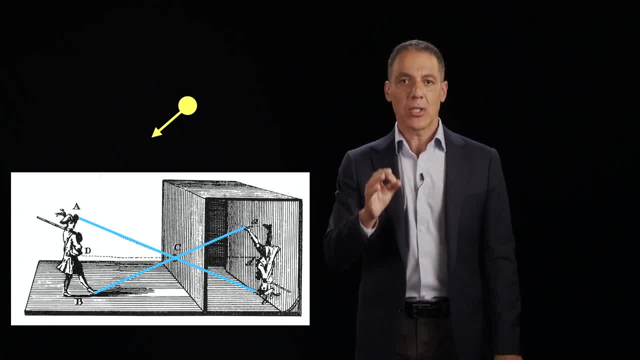 refrigerator box, seal it all up, go inside and you can see that the light is coming out of the back of the camera. And then you go inside of it, open a little hole and on the back of the side of where the hole is you will create an image. Many museums have these beautiful camera obscures. 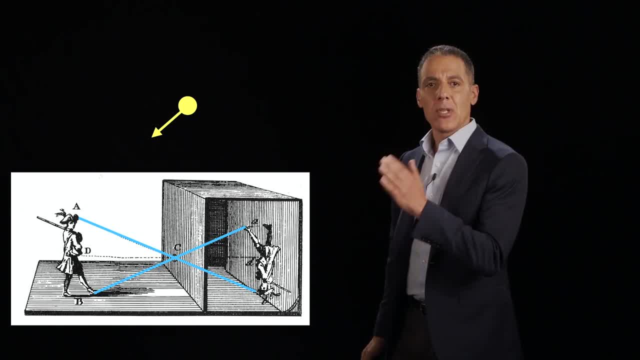 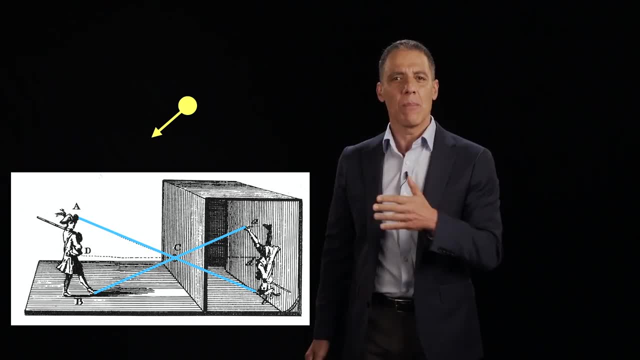 where you can see this image formation process. Now, what's missing here? Well, what's missing here is we're not recording the image. I mean, we're sort of recording it because it's in the back of the box, but we need something to record it more permanently, And so what we do is we slide. 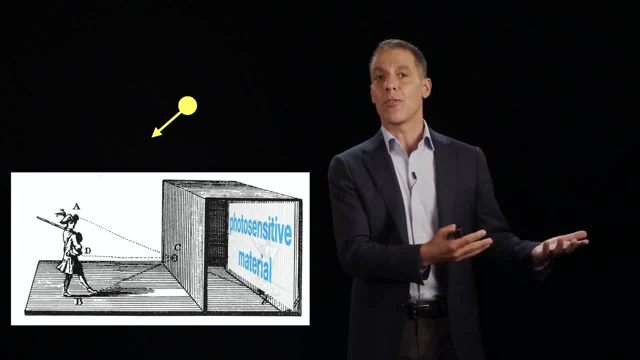 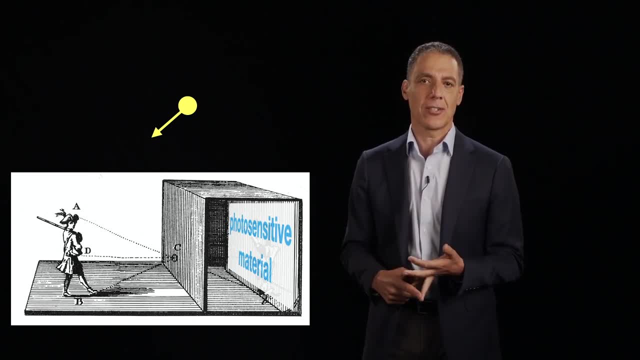 into the back of the box some photosensitive material- 35-millimeter film, Kodak film, for example. And these days it's a different type of sensor. It's a CCD sensor or a CMOS sensor that converts analog light into a digital signal. 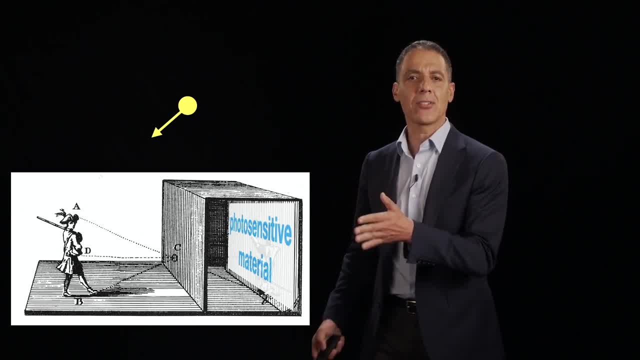 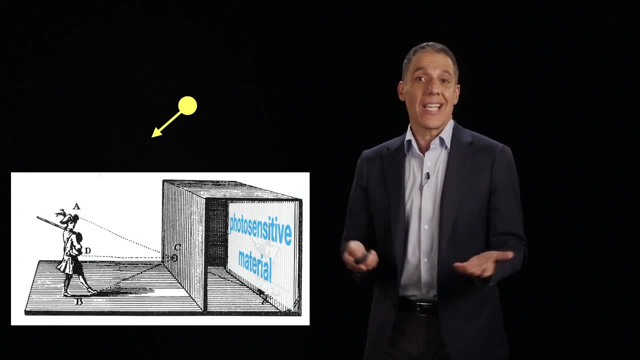 Whatever your favorite photosensitive material is, slap that in the back of the box and then, when light strikes the back of the box, the image will be recorded. And that is essentially what a modern camera does, but with some bells and with some whistles. 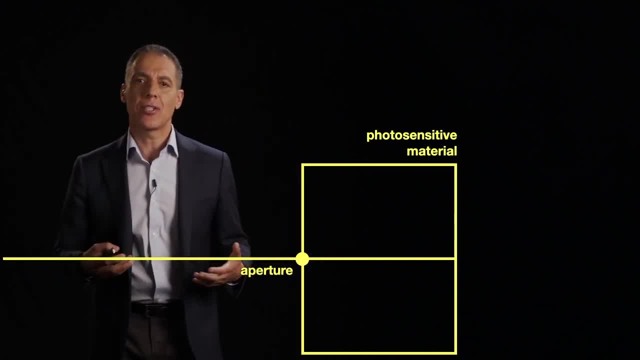 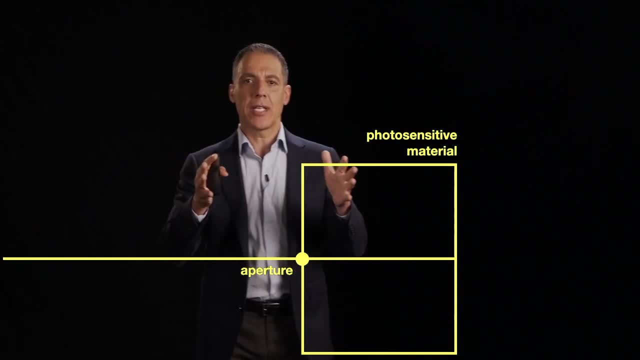 Now, throughout, We're going to need some nomenclature, So let me go ahead and start defining some terms that we're going to use over and over and over again. So first, this is my pinhole camera right here. It's just think about sort of looking down onto the box this way. 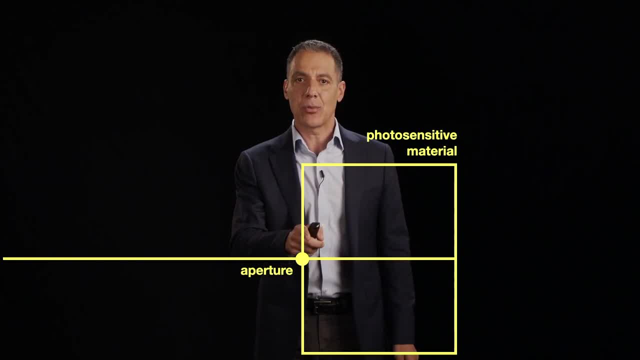 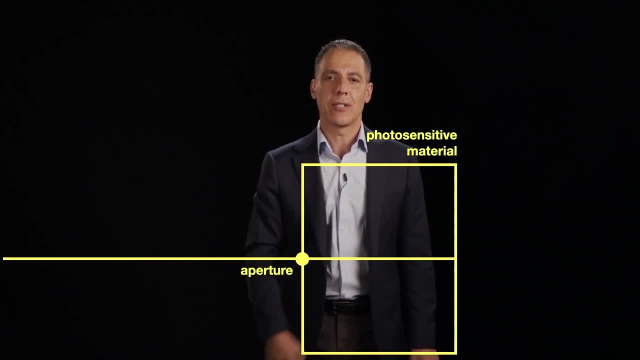 This is the top, This is the aperture. right there, That's that small little hole where the light went through, And on the back over here is the photosensitive material And I'm going to. So that's the photosensitive material there. 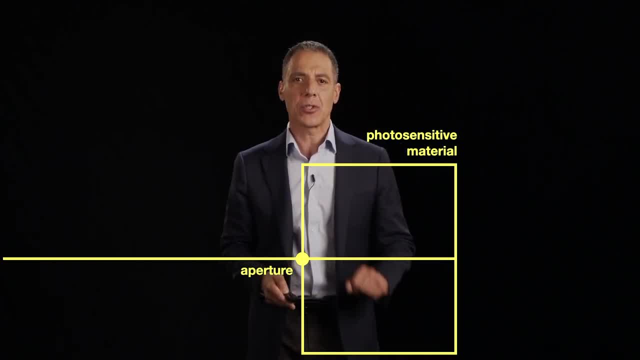 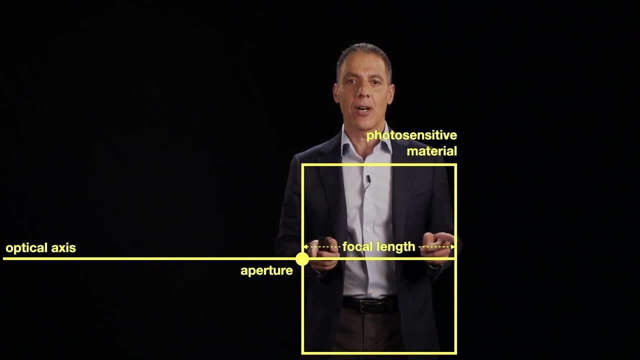 And we're going to define the aperture right here and I just need a few more terms to define. So I'm going to define the focal length as the distance between the aperture and the photosensitive material. I have control over that. I can make it small or large.